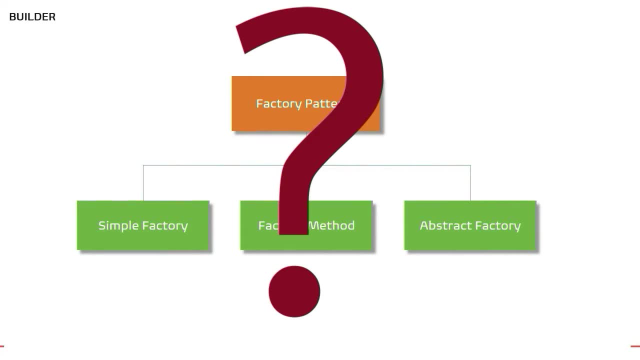 why other creational design patterns? This is primarily because the object creation might be complex, depending on the scenario. It is highly possible that if you don't choose the right way of creating object, then you might end up creating object in an inefficient way, which might be: 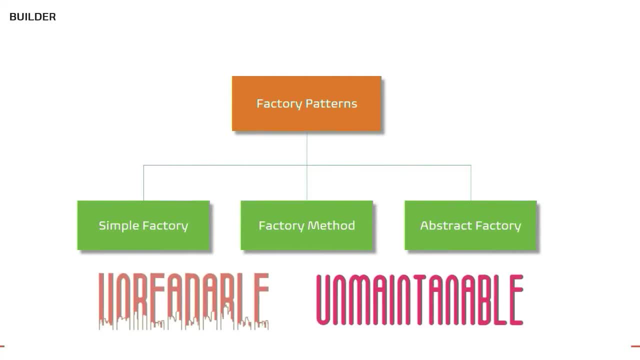 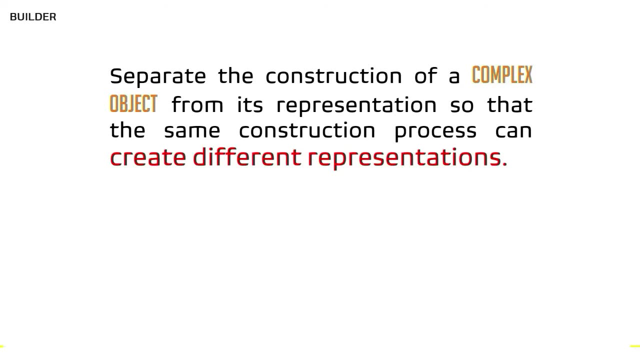 unreadable and unmaintainable, And this is one of the reasons why we have builder pattern. As per Gang of four definition, builder pattern is defined as separate the construction of a complex object from the structure of the object, And this is one of the reasons why we have builder pattern. 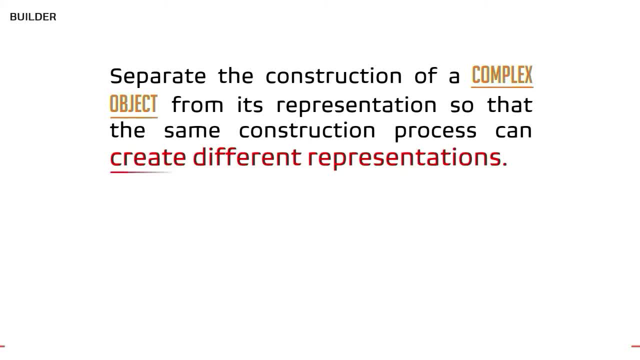 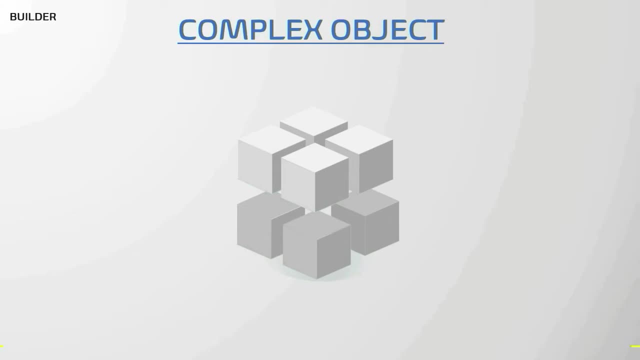 It is created from its representation, so that the same construction process can create different representations. I will explain this UML diagram Once we understand the initial bits and pieces of this pattern. Now, what do you understand by a complex object? Generally, a complex object is: 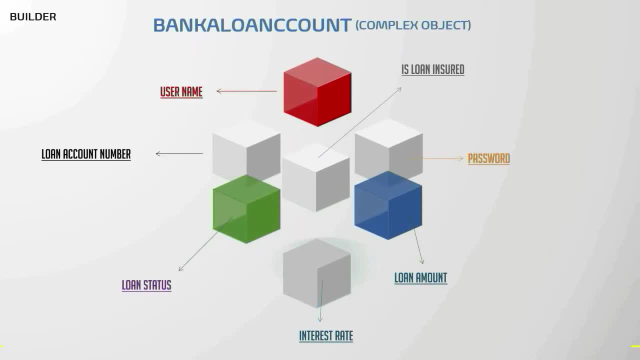 the one which are made up of multiple parts. Now, as you have seen here, loan account builder is our complex object. It contains the attributes like username, password, loan account number isLoanInsured, LoanStatus, InterestRate, LoanAmount, etc. 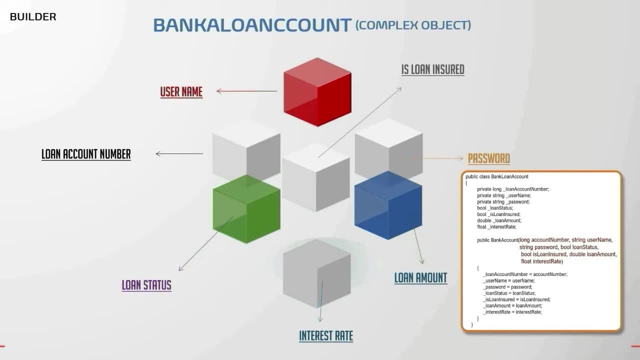 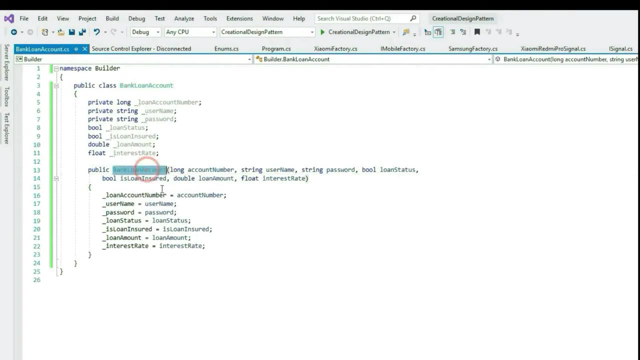 Or in plain coding terminology, it could be a class that receives multiple constructor parameters, which can at times increase or decrease. Please pay attention to the number of arguments here. Let me show you this in Visual Studio. So here I have a class called BankLoanAccount and only one constructor with several parameters. 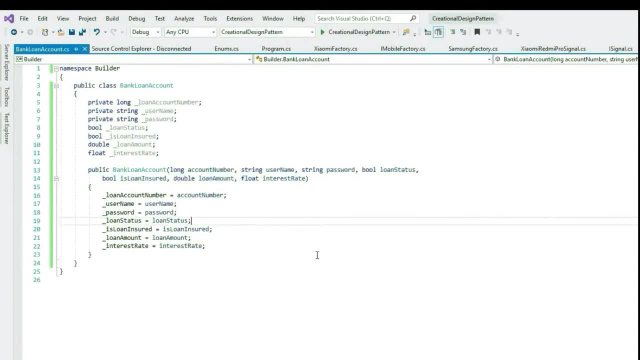 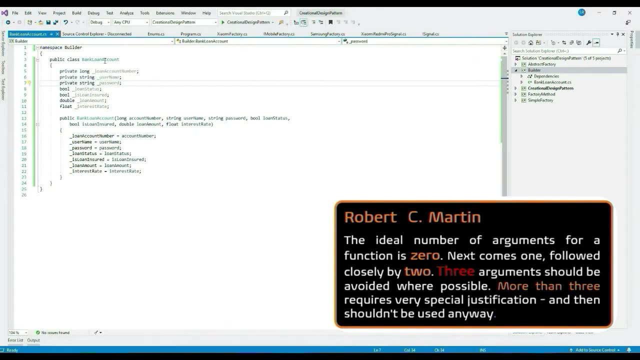 We know that any class that has more than three arguments creates code smell and hence not a good practice. As Robert C Martin has stated, the ideal number of arguments for a function is zero. Next comes one, followed closely by two. Three arguments should be avoided where possible. 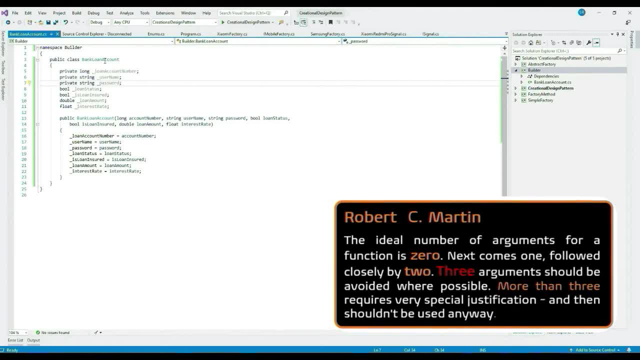 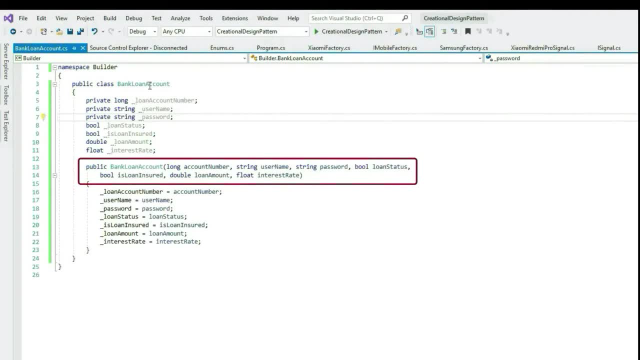 More than three requires very special justification and then shouldn't be used anyway In our case. these many arguments also clearly tell that any time these arguments can increase or decrease as well. Once these arguments increase, it will be extremely difficult for you to manage the 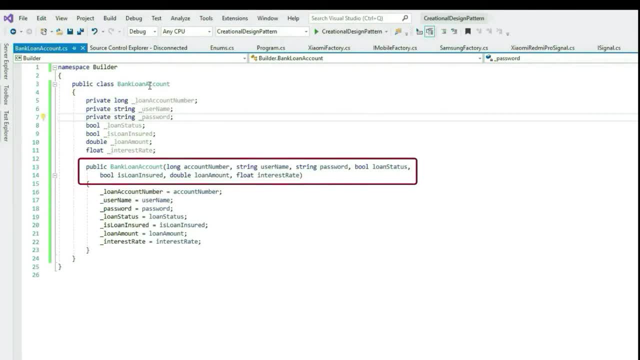 code, as it will adversely impact code readability. So this is not an efficient way of building this object, where we have a lot of parameters, and especially when we anticipate that the parameters might increase or decrease. Now let's come to the next part of the definition and see another scenario. 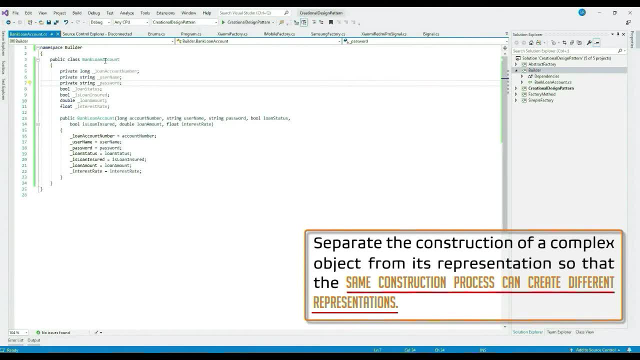 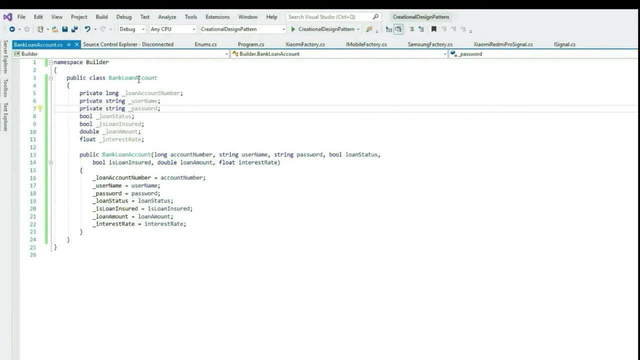 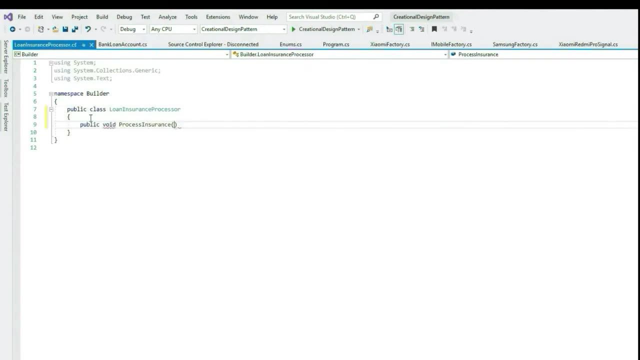 The second part says the same construction process can create multiple representations. Say you want to have a different text. Say you want to have a different representation of this class, Perhaps say you have another class called loan insurance processor. Let's quickly create that class. 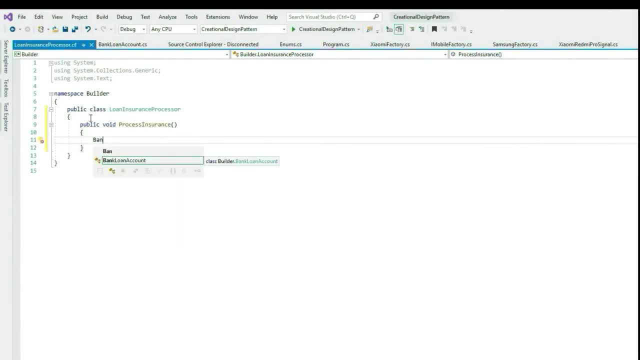 Now say, in this class you need an instance of bank loan account class. But this loan insurance processor class is interested to create the object with only loan account number, loan amount and isLoanInsured. Is this possible here? No, with the current design you cannot create separate representation of this class. 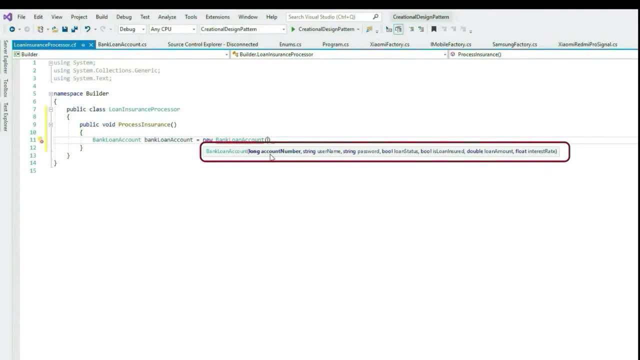 It means it has to pass all these parameters while instantiating this class. If the phrase separate representation of the class is confusing you at this moment, please bear with me for some time and everything will be clear. Let's go back to our slide. 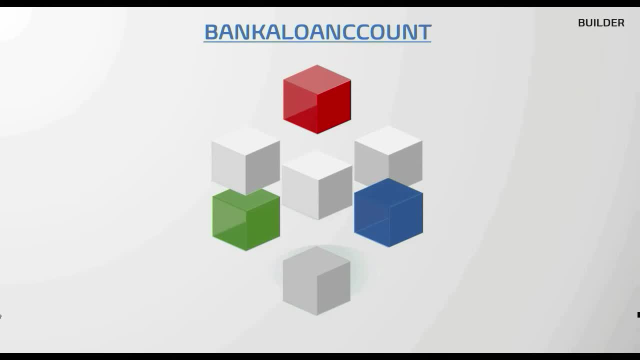 Let's assume this is your complex object. we have just seen Now how does builder pattern helps. The pattern can build the object part by part, joining all simple and needed parts together. It means it can pick the required arguments and can create a different representation. 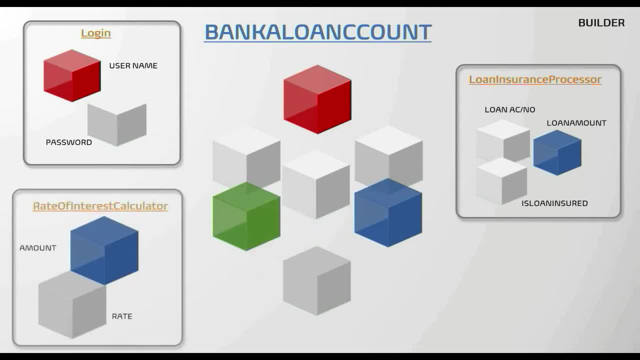 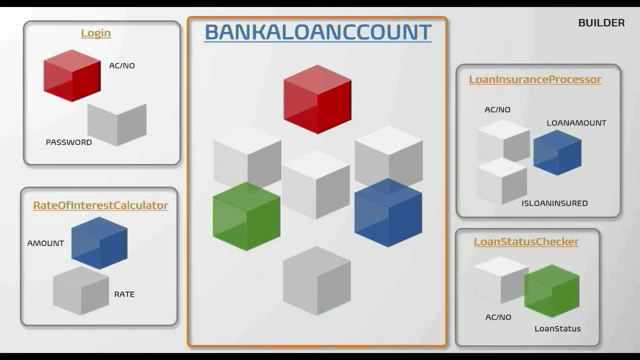 of it, Which ultimately means that it can instantiate this class with only required attributes. Here we had one class- bank loan account- but using builder pattern we can create more than one representation of it. Let's flip to Visual Studio and quickly look at it. 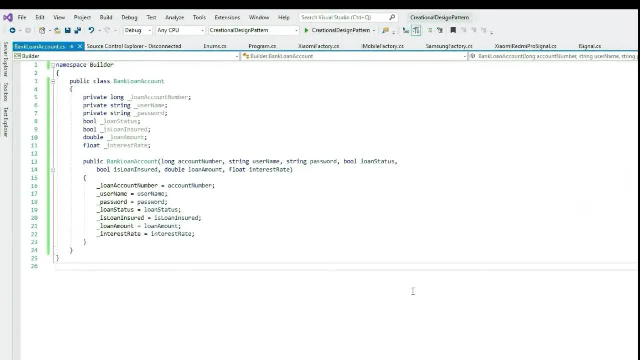 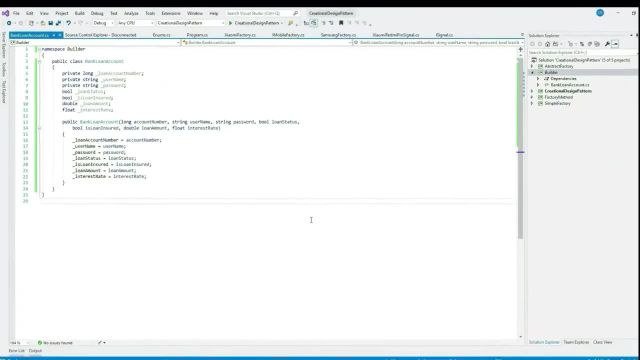 Here we have one class- bank loan account- but using builder pattern, we can create more than one representation of it. As you can see, this class has a big number of ever increasing constructor parameters, so this could be one of the use case where we can use builder pattern. 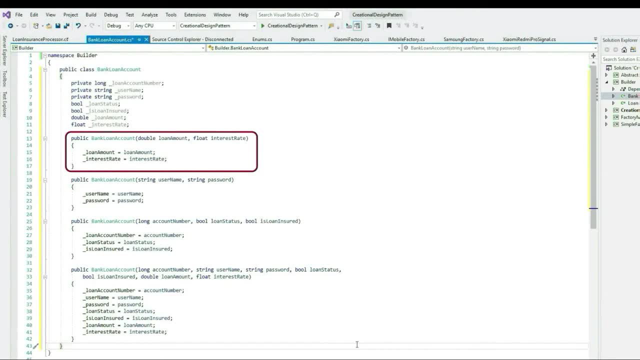 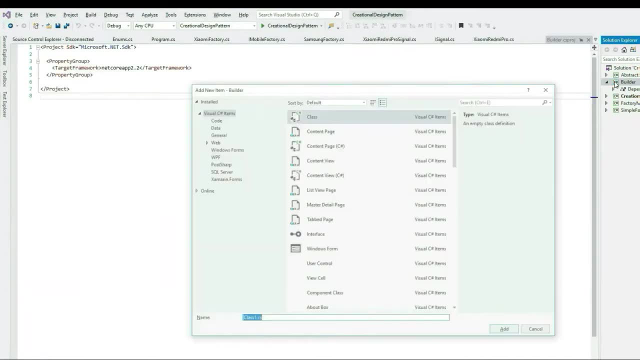 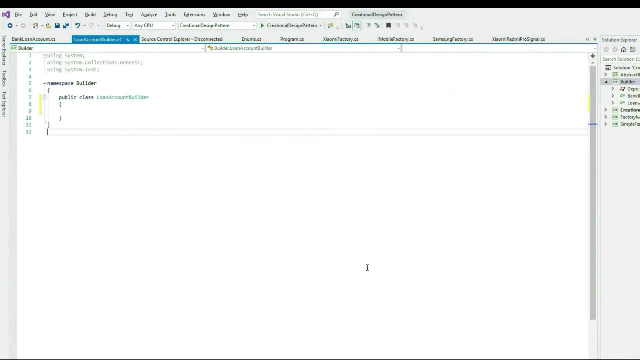 If this class would have been like this, with multiple constructor overloaded, then also it would have been a good contender. Let's create a loan account builder class. The idea is to go step by step or part by part and build a new object, Then start building. 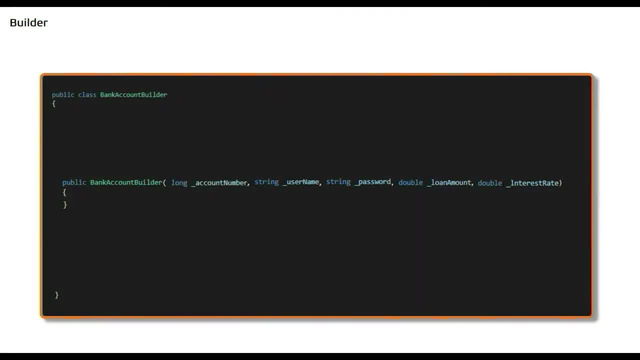 See how this class works with the required attribute. Now in factory we have the method parameters. With builder, all parameters will become a field and these fields will be set using a separate method. Builders, practically, are most often constructed using a self-referencing method. 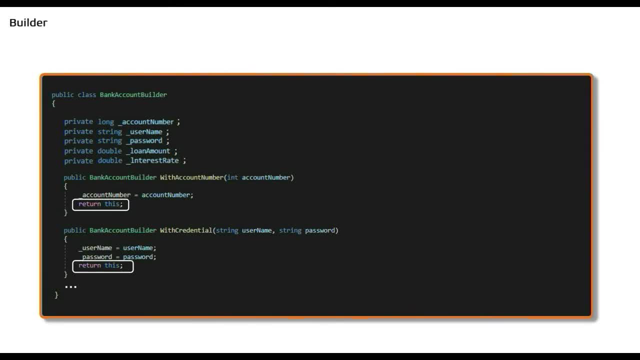 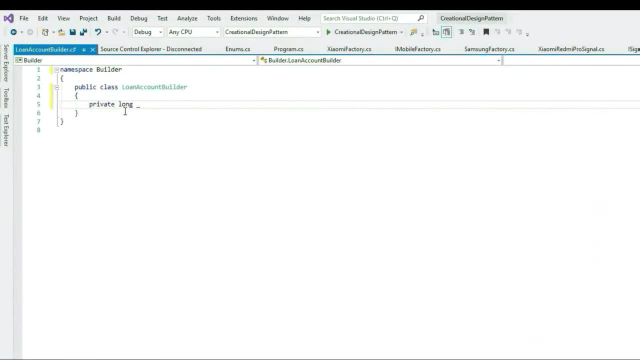 Hence the methods will return the same builder object so that next method can be chained. Let's quickly implement this. Let's create our private fields. to make things faster, let's copy and rename the fields. As mentioned earlier, this field will be set through a method. 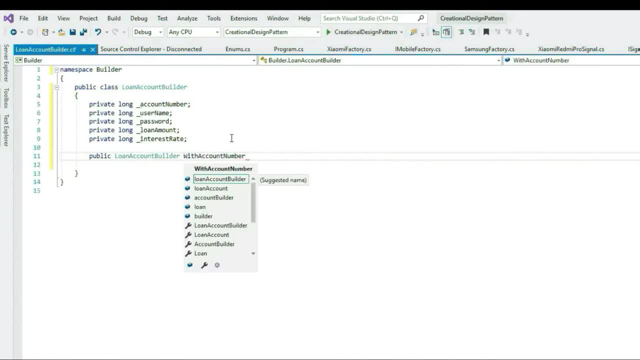 So let's create the appropriate method to set these fields. All these methods should return self, as these are self-referencing methods which will help us in method chaining later. Let's quickly create other required methods as well. Let's modify these to appropriate data type. 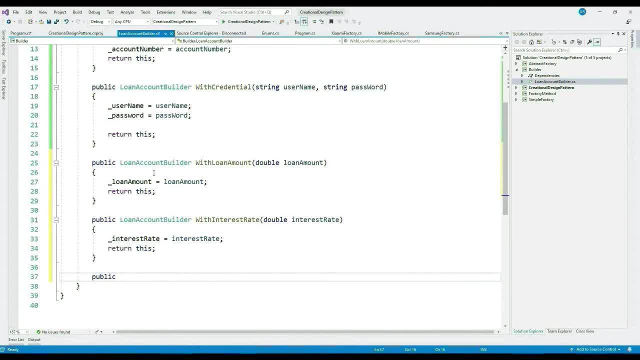 Finally, let's create our main build method, which will do this. Finally, let's create our main build method, which will do this. Finally, let's create our main build method, which will do this. Now let's return this object. 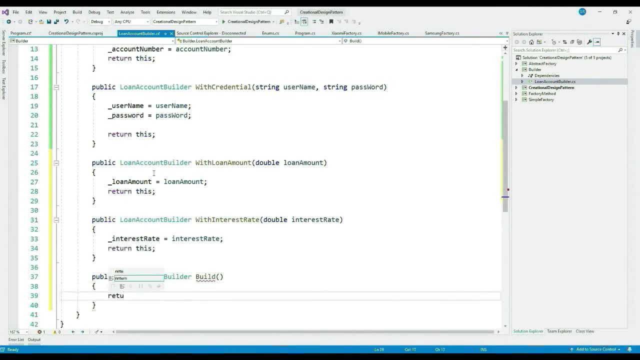 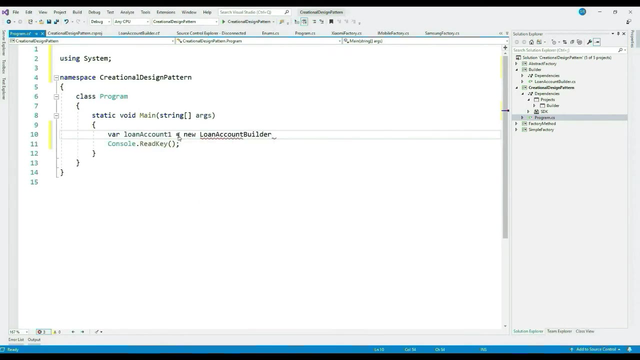 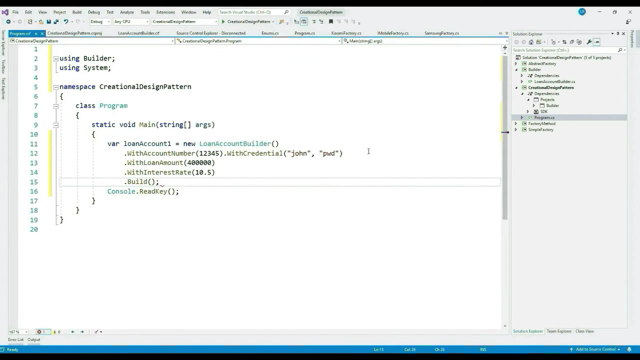 as per client's requirements. Let's add reference to our consumer application. Let's consume it at ConsumersEnd. Let's add the namespace. You can see we have all the methods here. Let's change only the required methods Here. our LoanAccount1 object contains all attributes, but we can always create LoanAccount. 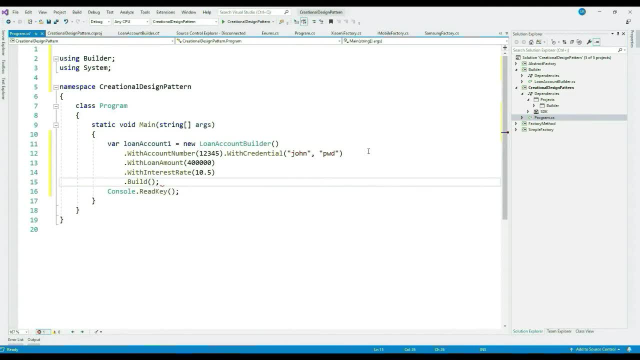 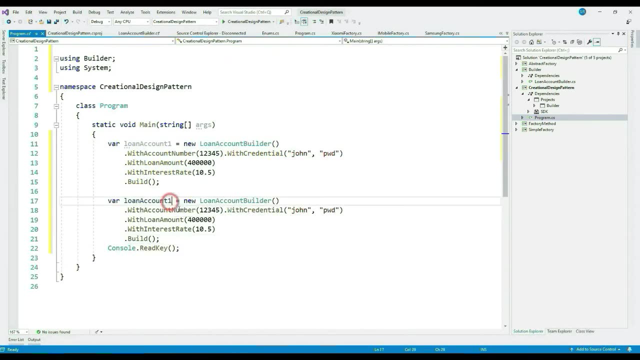 object with few required attributes as well. Let's create one such object. Let me copy LoanAccount1.. Let's create this object without credential. Now, this object is also completely valid, but contains only account number, loan amount and interest rate. I hope you have realized that, how you can create a separate representation of the same. 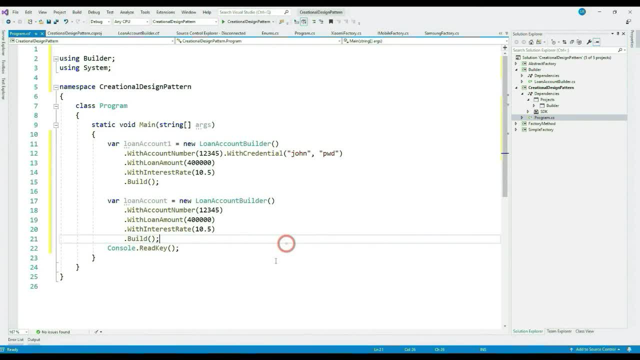 object. While creating object, there are certain things that you always need to take care, that is, should not allow invalid object to be created. That means we are yet to be done with the object creation using builder pattern. Let's add few validations. For instance, account number cannot be zero. 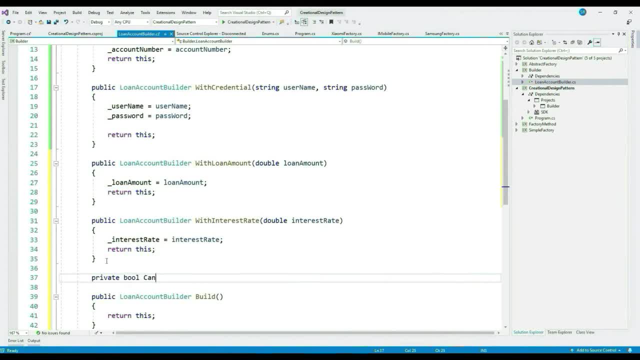 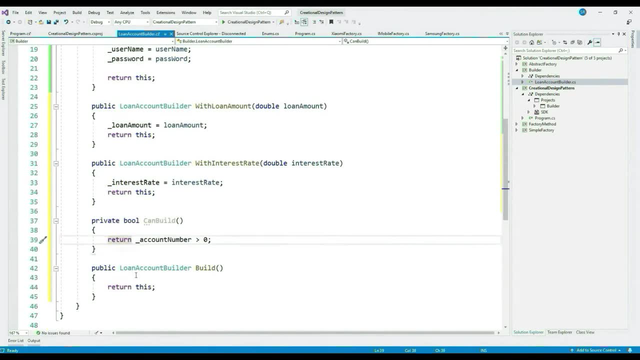 Let's create a private method canBuild to check that. Let's put the validation before returning the build object. Let's throw a general exception here with a message: cannot build a valid object. Let's build our class library. Let's create a private method canBuild. 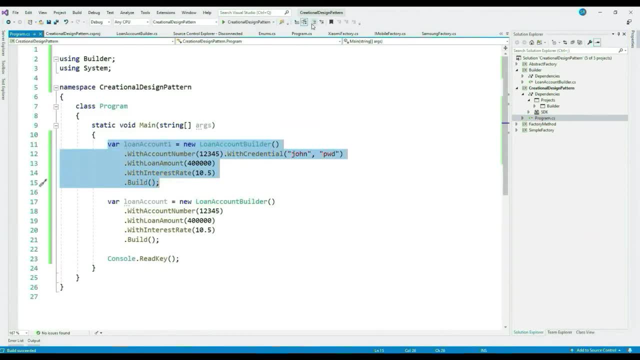 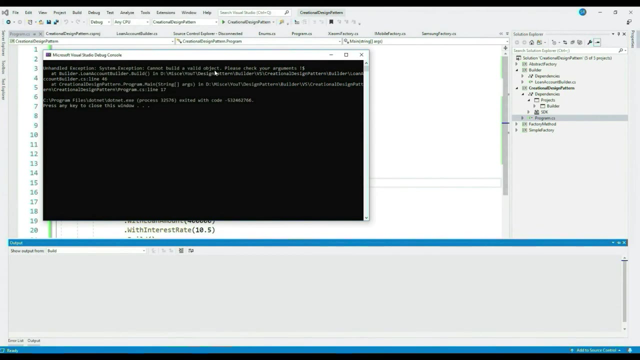 Let's see if our validation is working or not. Let me comment this and let me remove the account number from our object creation. Let me run this and see if it throws an exception. Yes, it throws an appropriate exception. cannot build a valid object. 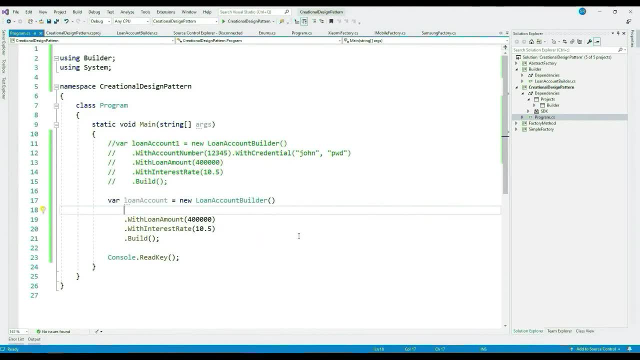 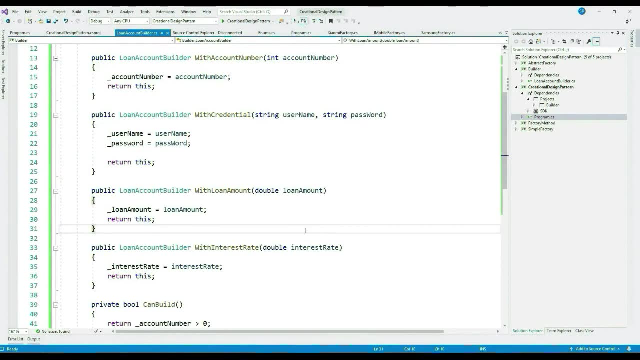 I hope you realize that how efficiently you can put your validation logic In fact you can even do per method validation. Let's see one more benefit of builder pattern. Now say you want to add one more attribute- loan status- to the object. 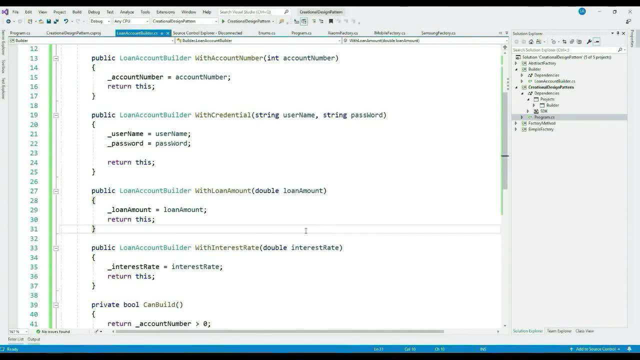 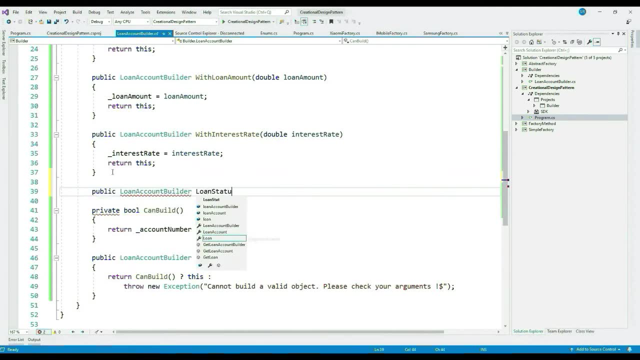 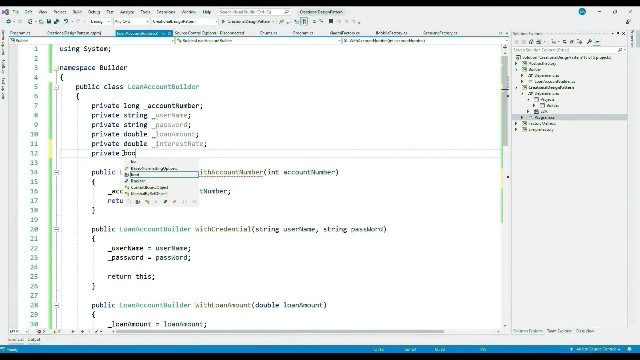 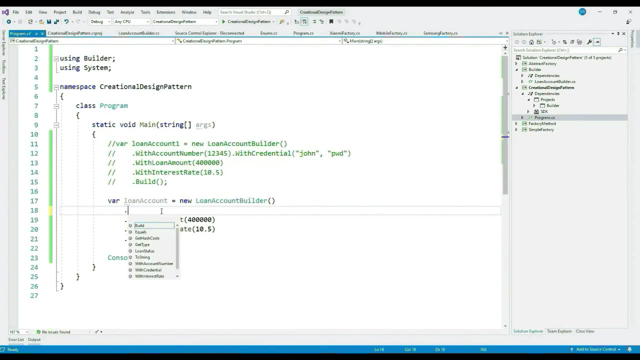 No problem, We can add it very easily. Let's see that. Let's create a self-referencing method For now. let's name it loan status. Let's create our private field. That's it. We can add this attribute to our object now. 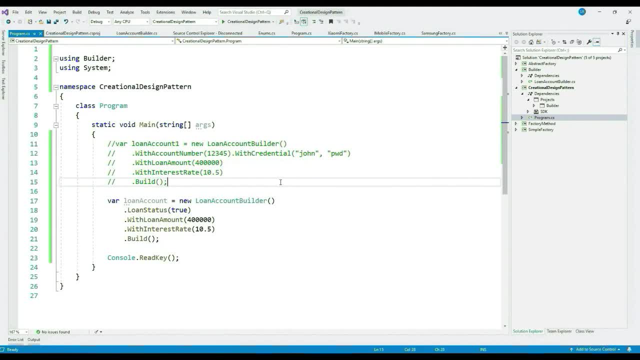 You can see how easy it is to add and remove attributes. now. This is the most common way of implementing builder pattern. However, this is not exactly like the way it has been done by Gang of four. I definitely wanted to explain the way it has been explained in Gang of four- UML- but 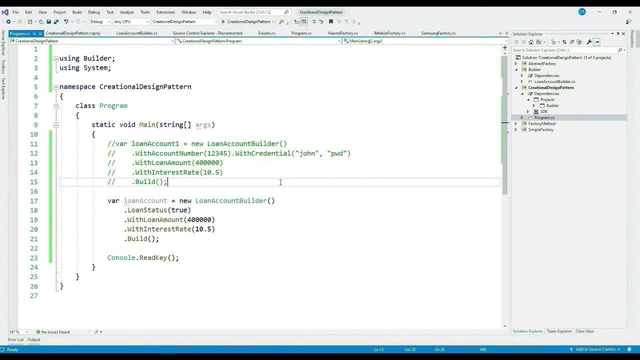 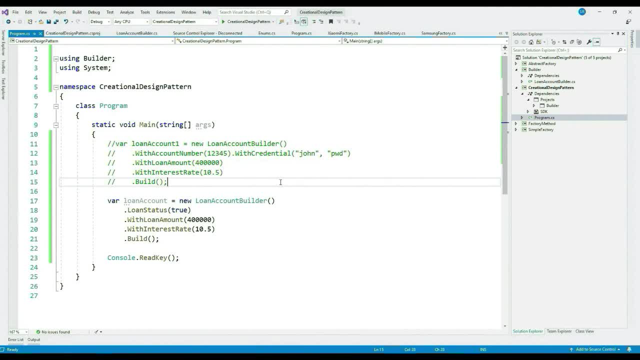 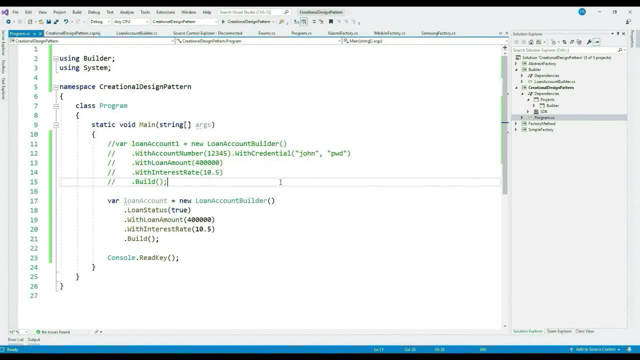 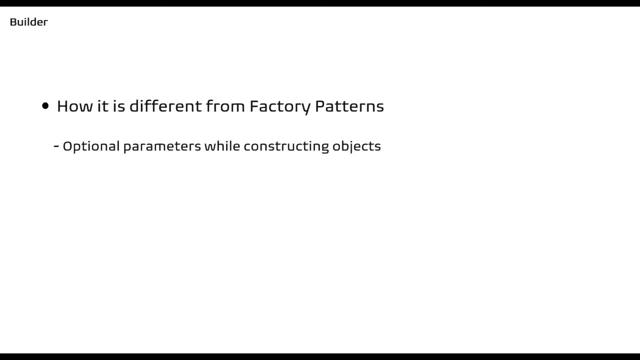 from factory and also list down when we should use this pattern. Factory patterns are good where they encapsulate object creation by decoupling the creation of the object and the consumer, But they fail to create the object when the construction process varies a lot. 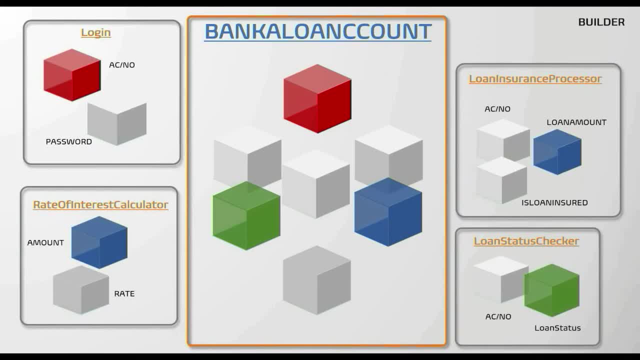 For instance, in our example, for most of the classes some of the parameters are given are optional. like for loan insurance processor, we require only three attributes. but since factory receives fixed signature, if we use factory we are forced to send all these parameters. it means factory method cannot create a. 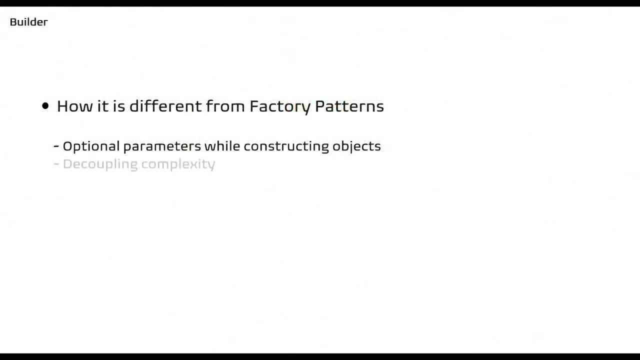 different representation of the object. if the object is heavy and its creation is complex, then all the complexity will be part of factory classes. at times this might be confusing, so we can consider using build a pattern here. I hope it is clear to you that even after having factory patterns for creating an object, 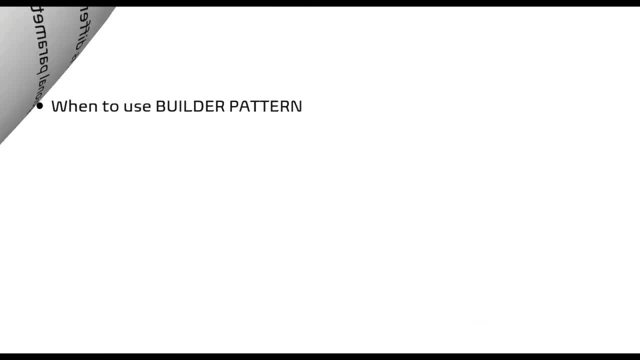 why we have built a pattern. so let's quickly discuss when to use this pattern. I would like to repeat here what I always say: do not try to use a pattern because you know it. only use it if it completely fit to your solution. because I believe that it is always tempting to implement the design pattern. 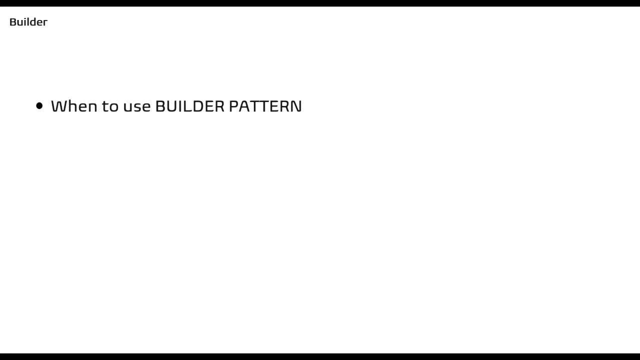 if we know it, even if it does not completely suits to our requirement, and when it comes to build a pattern, it is one of the pattern which has specific use cases where to use, most often, abstracting interface using other design pattern might solve your problem. having said that, let's quickly see when to use. 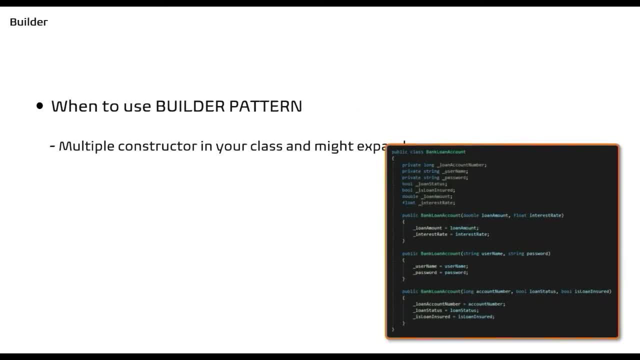 this pattern. if you have a class in your application that has multiple constructors and you anticipate it might increase as well, then it's highly possible that build a pattern suits to your solution, because multiple constructor means multiple representation of the class and, as we have seen, build a 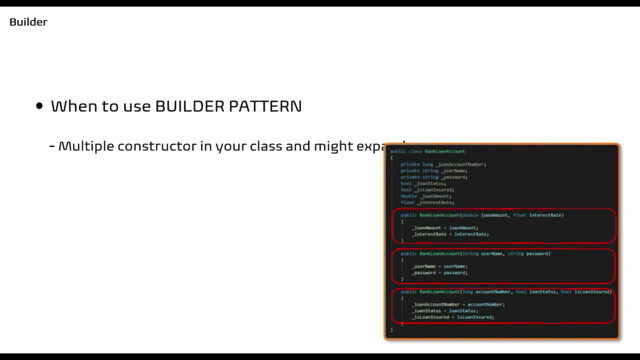 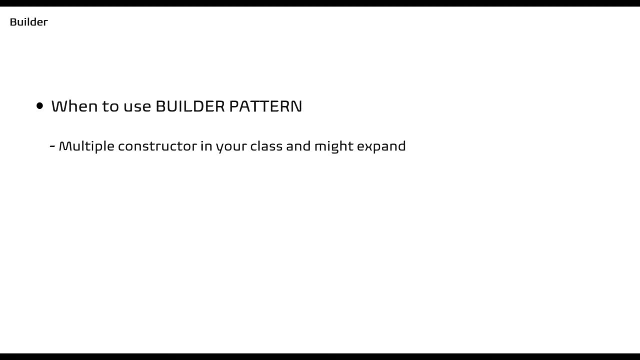 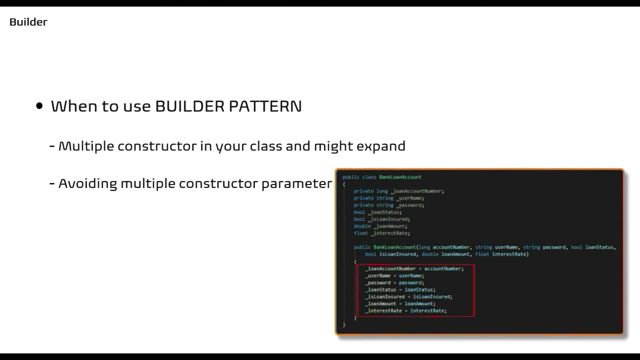 pattern helps in creating multiple representations. hence that's the time when you should consider refactoring your class with builder pattern. another use case would be when you have multiple parameters passed by a constructor and you do variety of computation before setting up the fields. then you can use.